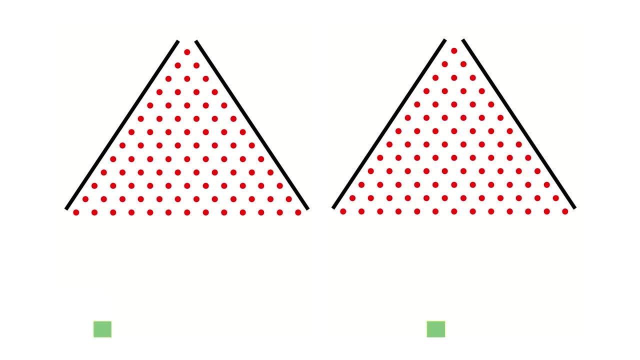 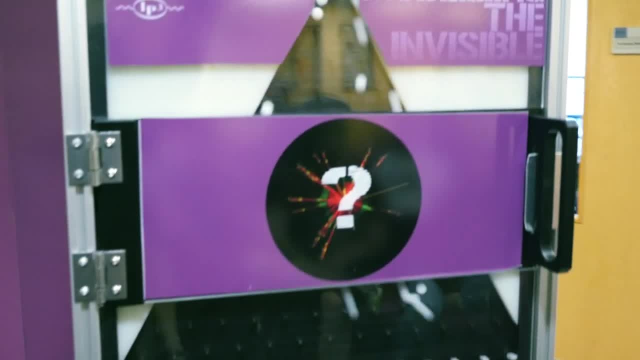 to running this experiment once and we don't learn much. We need more information. so we drop many more balls down and study the pattern formed in the tubes. We can see that there are more balls in the middle tubes than the outer ones, in a shape known as a bell curve. 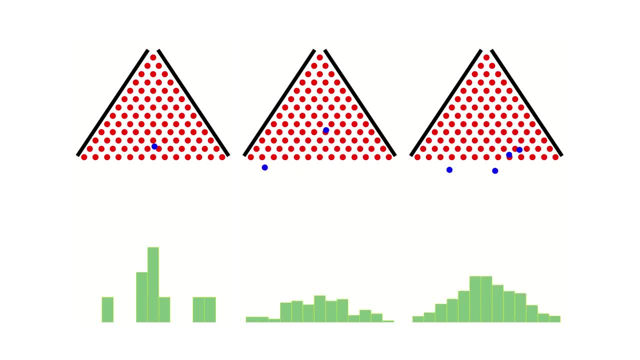 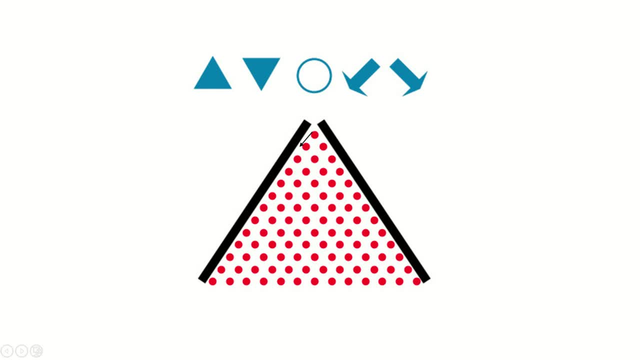 or normal distribution? We now have an answer to our original question. The balls are more likely to fall into the middle tubes than the edges. This is because, to land in an outer tube every time a ball hits a pin, it must go the same way, so there is only one. 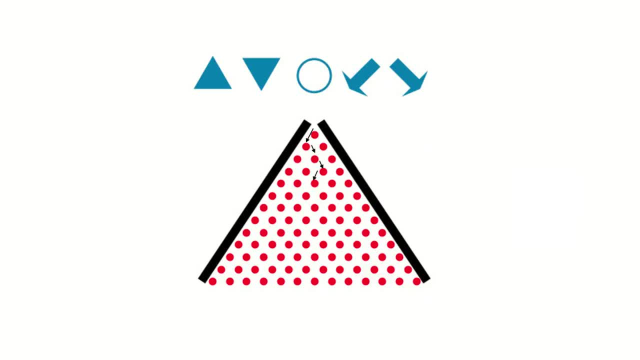 path that it can follow For a ball to land in one of the middle tubes. there are many possible paths, and so there is a higher chance that a ball will end up in the middle tubes. This is because the ball will fall into the middle tubes, and so there is a higher chance that a ball will end up in the middle tubes. 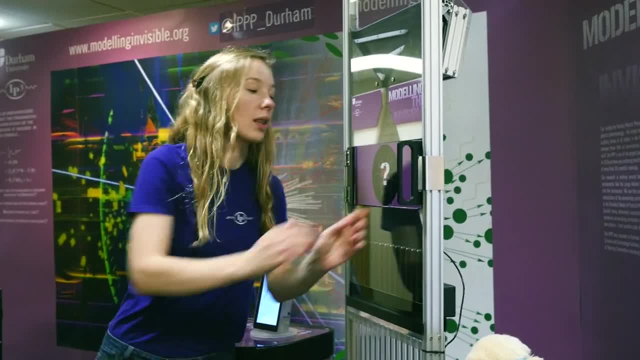 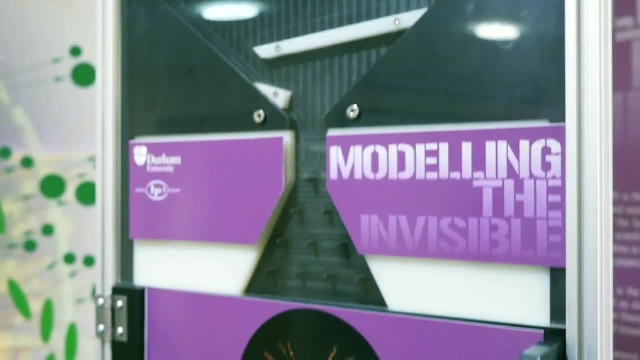 With this golden board, however, we can't see all the pins. How would we know if there is some sort of obstruction in the way or what shape that obstruction is? We have to work this out based only on the shape the balls create in the tubes. Again, we need 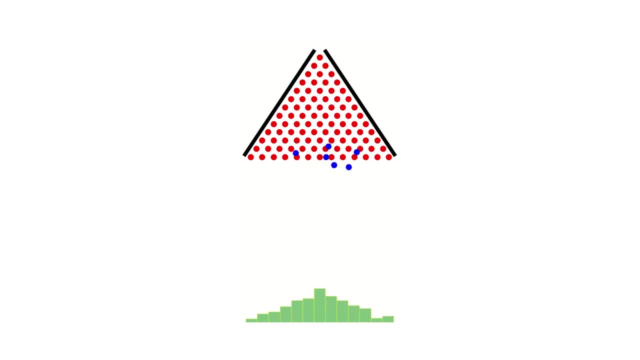 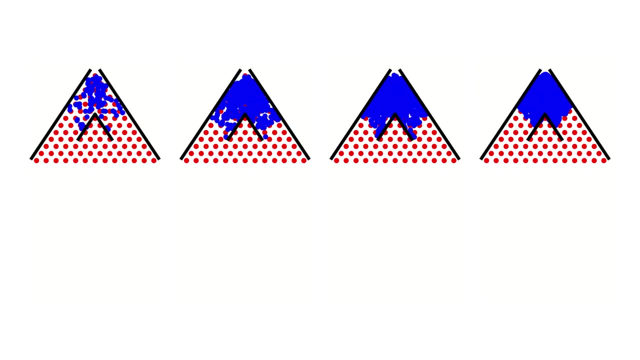 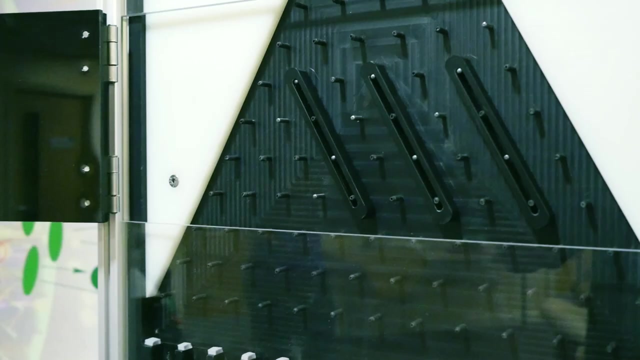 to drop as many balls down as we are able to. We can look at the pattern, and we may be able to understand some basic properties of the obstruction, for example whether it is symmetric. To understand more, though, we turn to computer simulations. Recreating the experiment as a computer programme allows us to model what is behind the door. 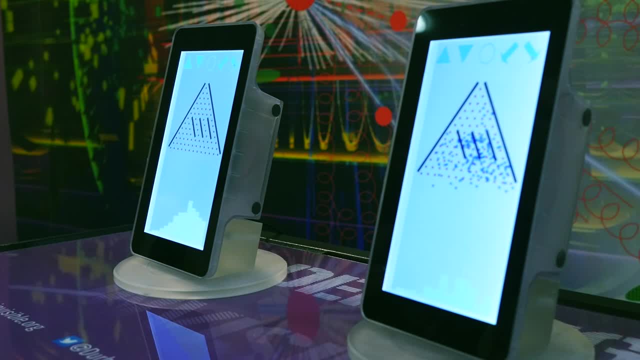 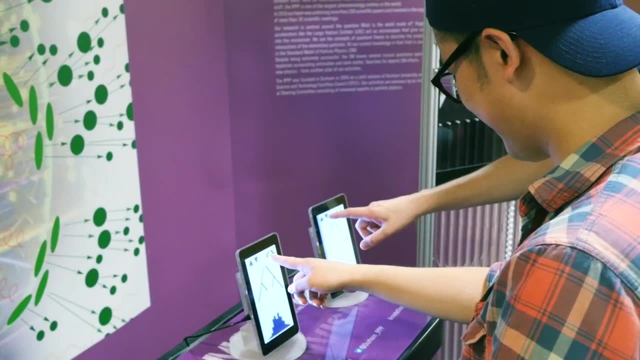 In the case of our golden board, we have five different options Running each option gives us a pattern similar to the shape of the balls in the tubes. By comparing the patterns we can determine which shape we think has been placed in the golden board. The patterns may: 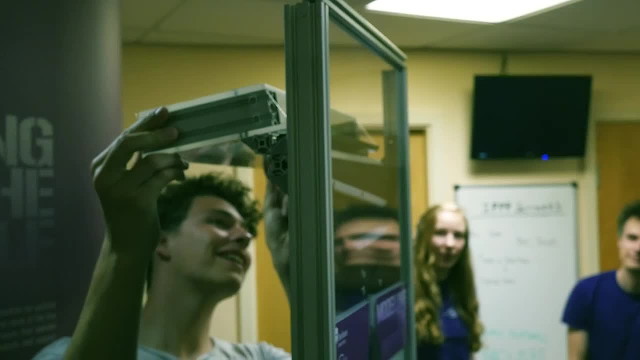 not match exactly, but running both the experiment and reducing the Carl's equation will allow us to determine which shape we think has been placed in the golden board. We don't can else. experiment and the simulation with more balls will improve the results and we can be more confident. 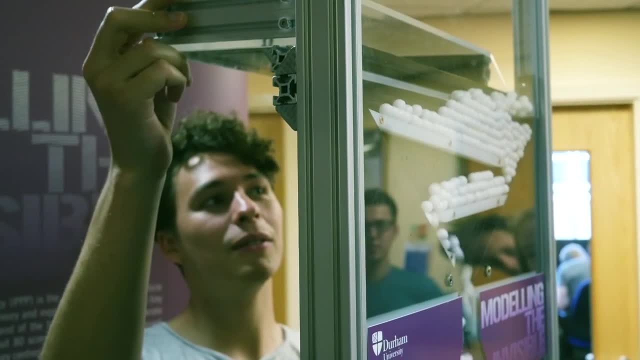 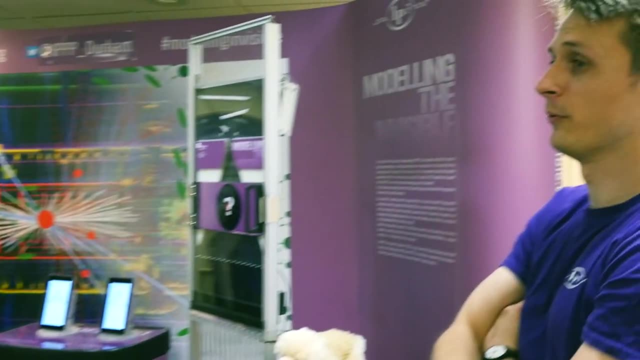 with our prediction. Of course, there is also always the chance that it is a completely different shape altogether, but it may only be with a lot more data that we would realize this. The Galton board is a simple example of a general principle. Often in science we are confronted with data that has